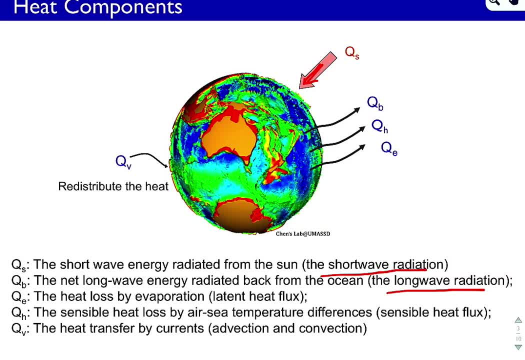 also known as backscatter. We have the evaporative heat flux, or latent heat flux, and we have the heat flux that's due to air-sea temperature differences, that drives heat across the gradient, and that's known as a conductive or sensible heat flux. So those form a one-dimensional balance and 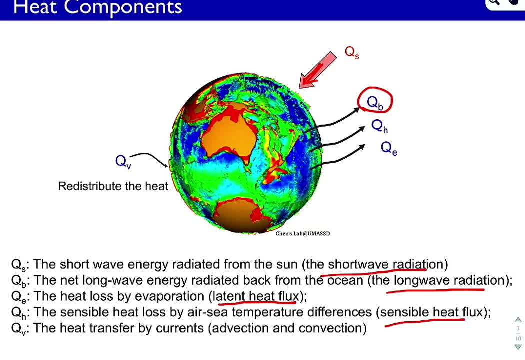 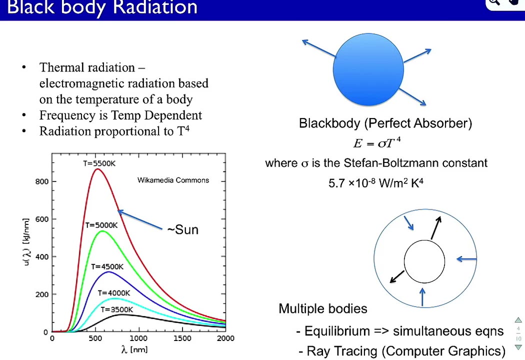 then the oceanic heat content is also distributed around the earth by currents that carry warm water, various places. For example, the Gulf Stream transports a very large amount of heat northward and allows places like England that are fairly high latitude to be quite warm. The solar radiation is: 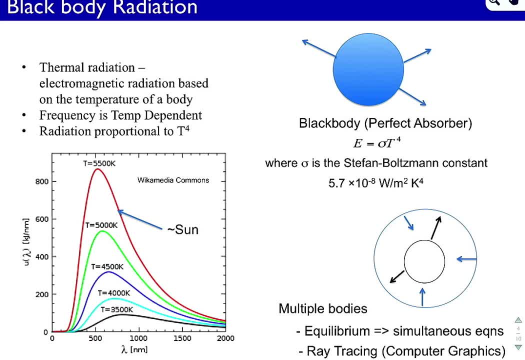 a form of blackbody radiation. All bodies with a temperature greater than zero Celsius give off radiation. This does not require a medium. Radiation can move directly through space, as it does from the sun. The radiation that a body gives off is dependent on the temperature of the body. In fact, it's proportional to the temperature of the body. 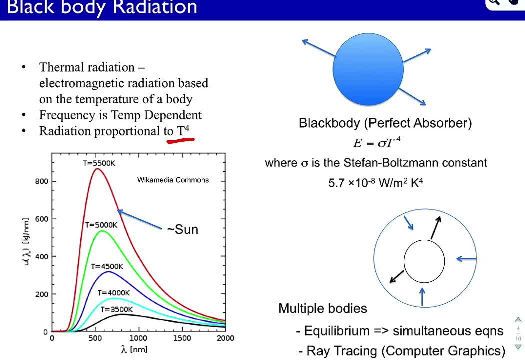 to the fourth power. The greater the temperature of the body, the greater the radiative energy given off. The exact formula is given by the Stefan equation here. It's proportional to the temperature of the fourth, where the constant of proportionality is the Stefan-Boltzmann constant provided here. 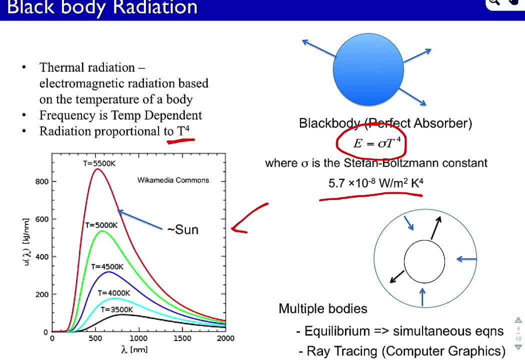 The spectrum of the radiation also varies with temperature, and here we have the wavelength in nanometers of the energy. 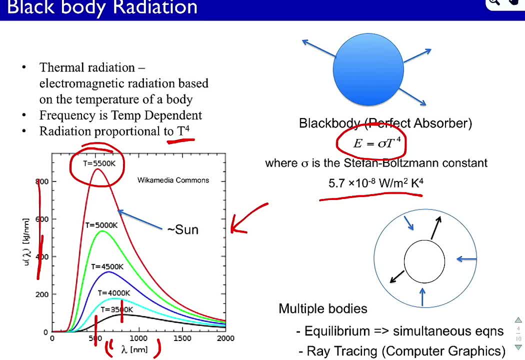 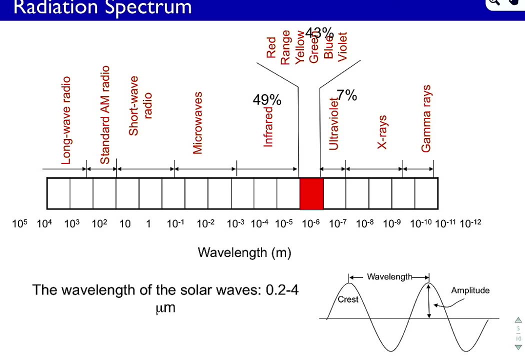 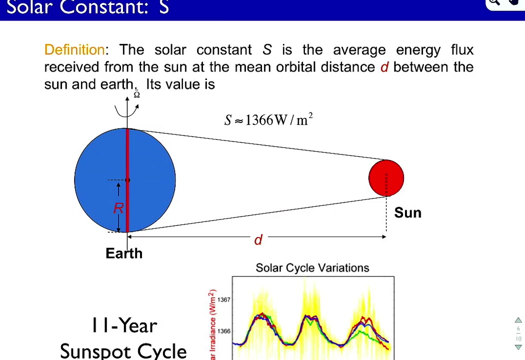 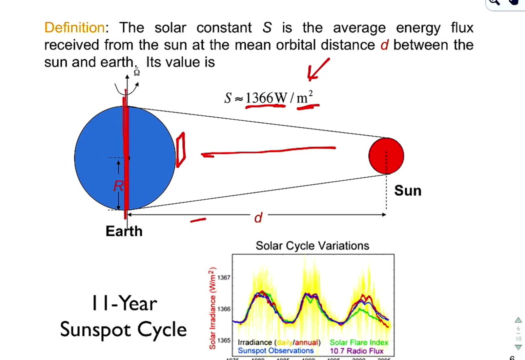 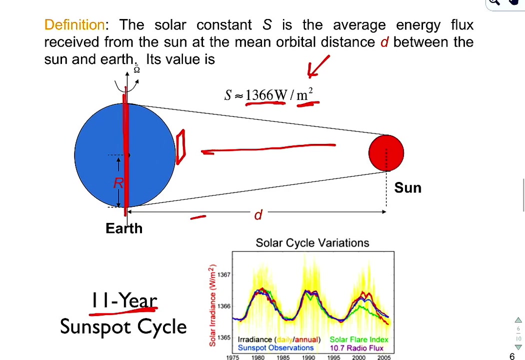 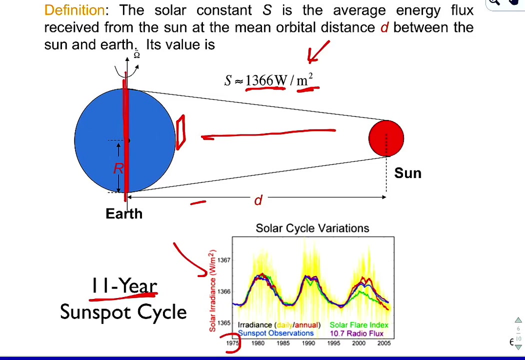 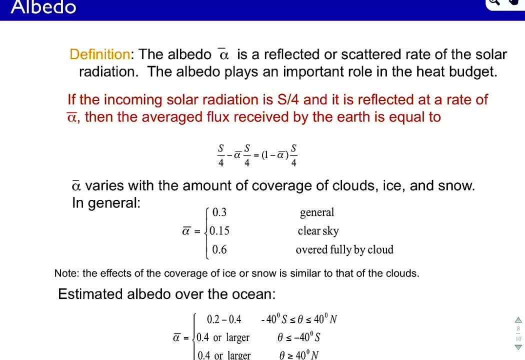 Reflecting off the clouds, reflecting the atmosphere as a whole. That reflection we quantify using what is called the albedo. The albedo is essentially the fraction that is reflected or scattered of the solar radiation, and it varies over the planet. it depends on cloud cover on the earth. that depends on. 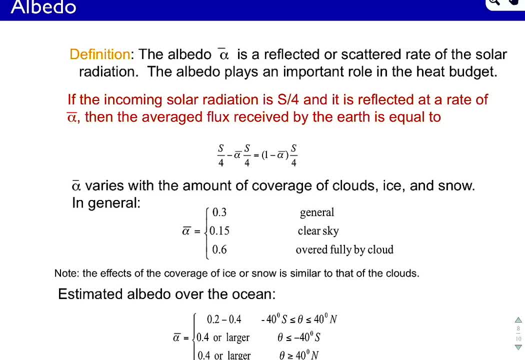 what's covering the. the local area, for example, of Snow has a high albedo. Ice has a high albedo. places where light reflects easily. The desert has a high albedo. Water has a relatively low albedo. Water likes to soak up solar radiation. 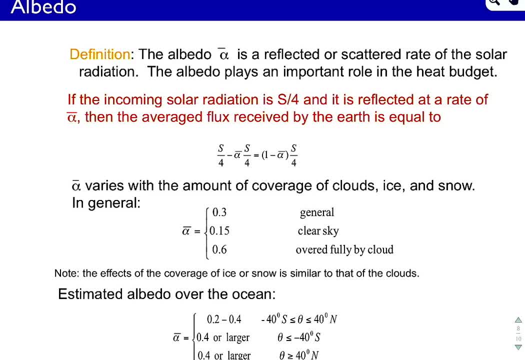 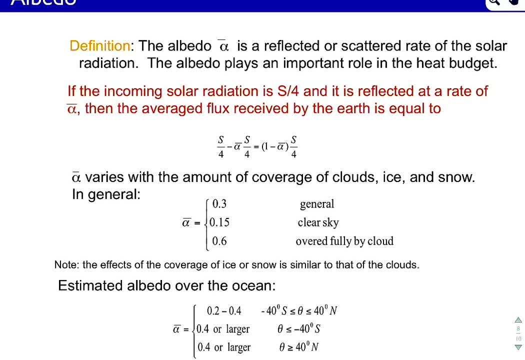 So there are variations depending on if you're over water or if you're over land, and if that land is covered by snow, ice or sand, And places that have persistent cloud cover on the planet are going to have- like some places in the tropics are going to have- a higher albedo. 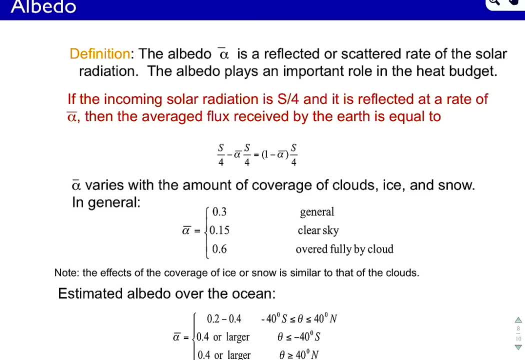 because much of the sun's energy is reflected directly off the clouds back into outer space. It never reaches the planet, It's not available for heating the planet. So these you can see the variations here of this albedo, the highest being due to cloud cover here. 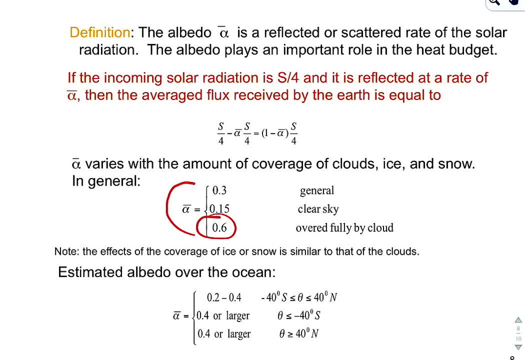 And these kind of variations occur latitudinally, due to ice coverage and cloud coverage primarily. On average it's about 50%. You can think of an albedo. the amount of solar radiation that actually gets to the planet is about roughly 50%. 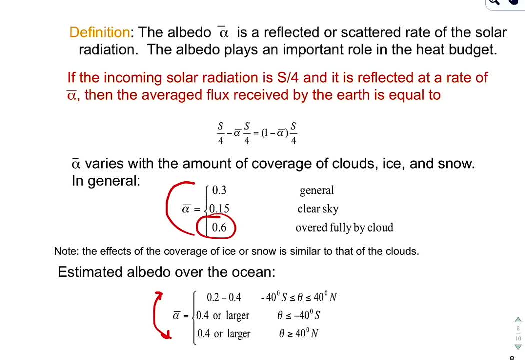 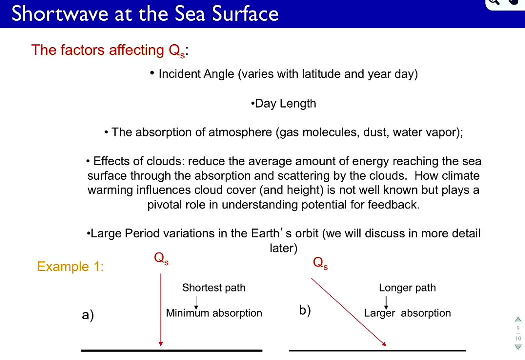 But it does have strong latitudinal and seasonal and even longitudinal variation, depending upon those factors I discussed Now, thinking in terms of latitudinal or variations in the incident shortwave at the Earth. so on average we get S over 4.. 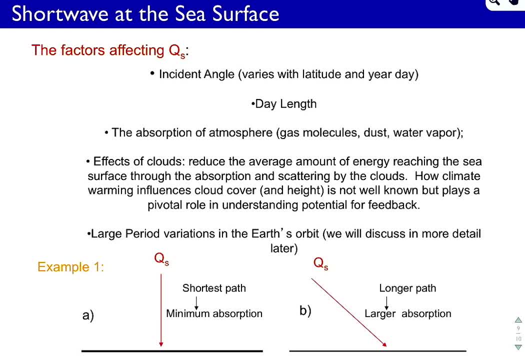 That's what we determined. We determined using simple arguments. At a particular location, you may experience more or less than that S over 4, depending upon key factors. One is this incident angle of incidence, and this has to do with what latitude you're at. 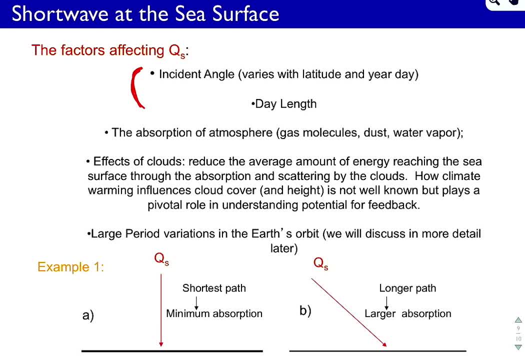 Areas near the equator are going, on average, to receive greater than S over 4 solar radiation than those at the poles. Local absorption from the atmosphere, depending upon the composition of the atmosphere nearby, effects of clouds, et cetera, as we discussed. 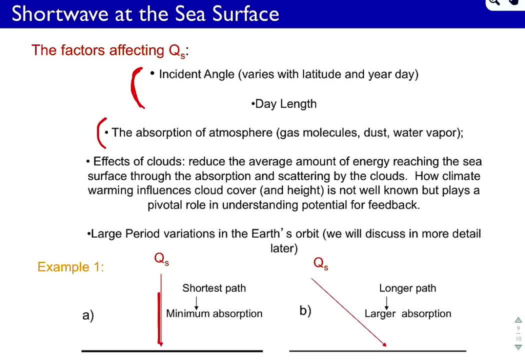 So the minimum, so you get the shortest path if the sun is directly normal to the land. So if the sun is directly overhead, you have the shortest path from the sun to you. You are most likely at that point to get a sunburn. 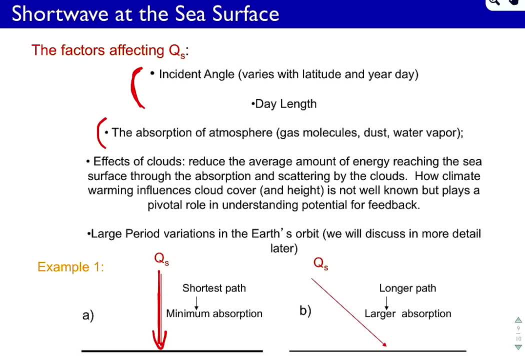 That is because you have minimum absorption of the solar radiation coming down onto your body. You also have the greatest amount of solar radiation regionally, Reaching a meter squared available for the meter squared At higher latitudes or when the sun is lower on average in the sky. 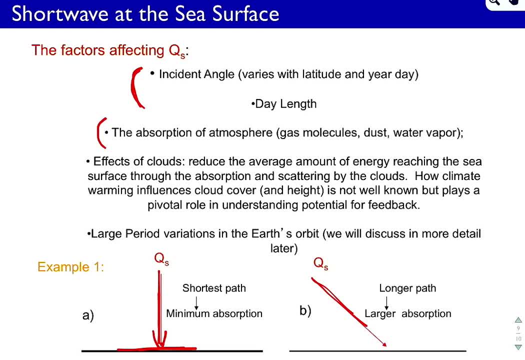 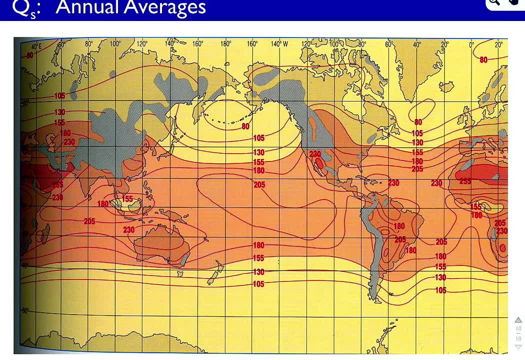 you have. the sun has to traverse a longer path and therefore has larger absorption to the atmosphere. When we look at annual averages, you see the most. the strongest effect here is the- excuse me, is the latitudinal variation. So you have the strongest a band of the strongest sun in the interior here. 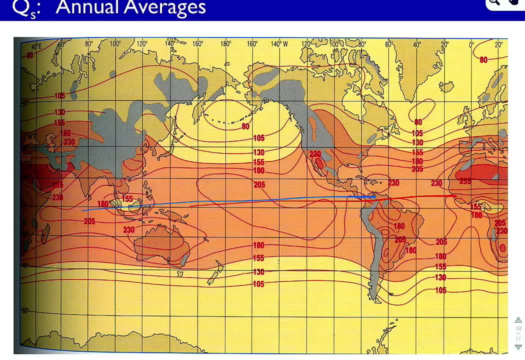 And you can see we're getting 250, something like that. watts per meter squared: Uh, 255 is roughly the peak that I'm seeing here, maybe a little bit higher And again, so you have your s over 4.. That's the average received by on the planet. 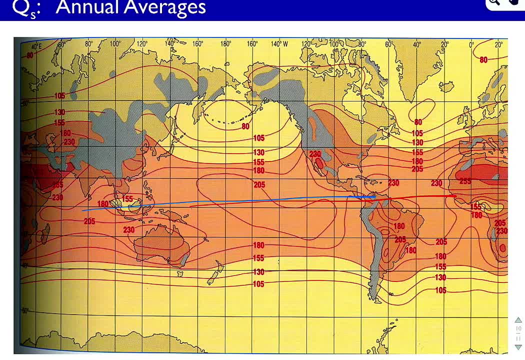 And then you have the albedo effects acting on to reduce that s over 4 further, down to a peak of about 300 watts per meter squared, And when you get to the polar region it's under 100 watts per meter squared because the sun is so low in the sky for at least half the year. 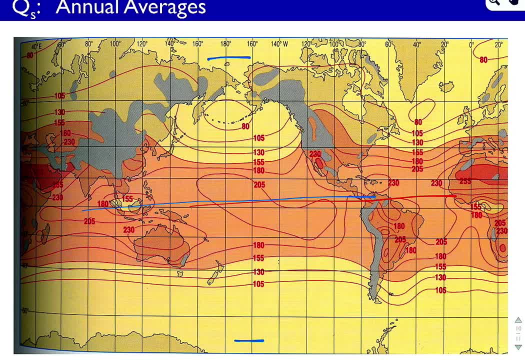 So we have- these are again annual averages, So you have strong latitudinal variation and you have some longitudinal variation. You can see that the contours tend to bend up Or bend away from the equator as they approach the land. So the contours are coming up to produce higher solar radiation over the earth, over the continents, than over the ocean.